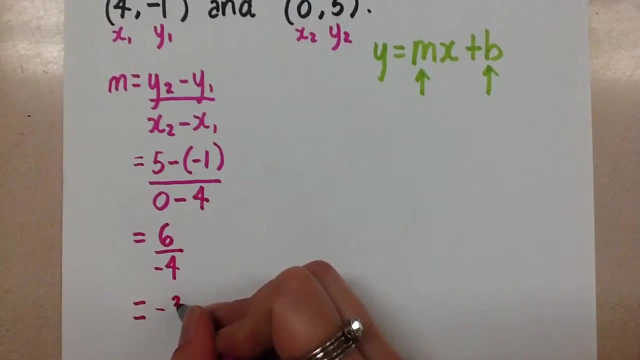 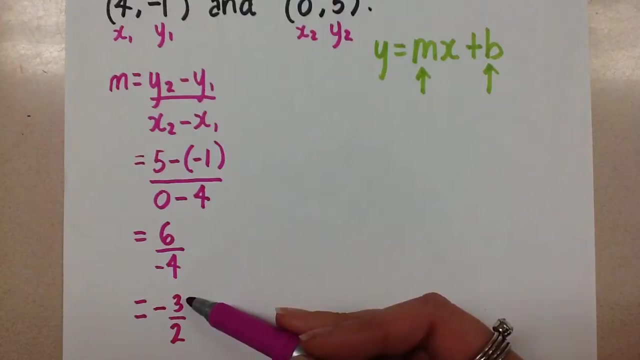 and that will give us negative 3 over 2.. You can use a decimal if you prefer. That would be negative 1.5.. That's up to you, but we always prefer the reduced fractions, especially when we're talking about slope, because then, if we wanted to graph this, we have the rise. 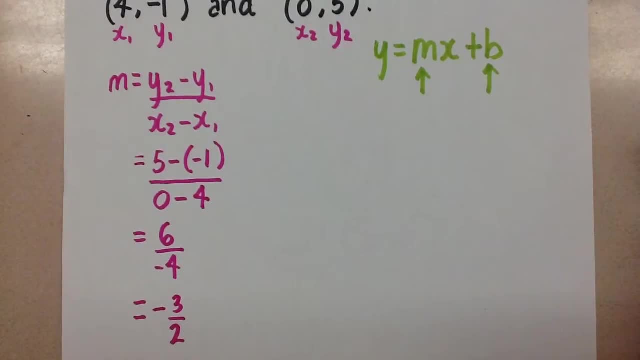 and the run clearly indicated in that fraction. So there's our slope. So we have now a slope and we're going to use the same process that we use when we have a slope and a point to figure out the y-intercept now that we need. 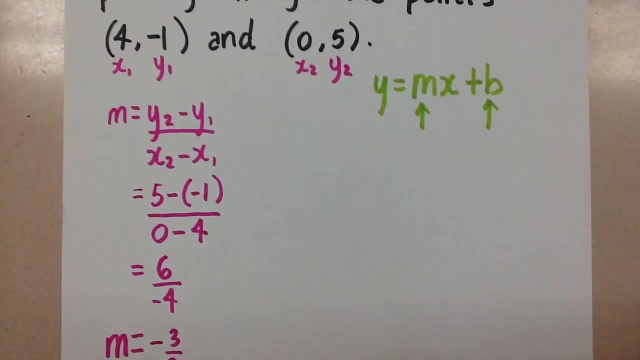 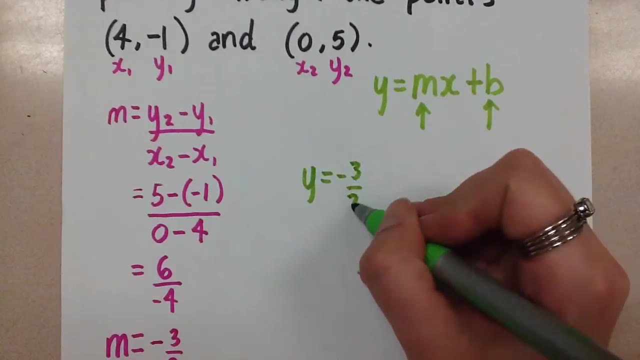 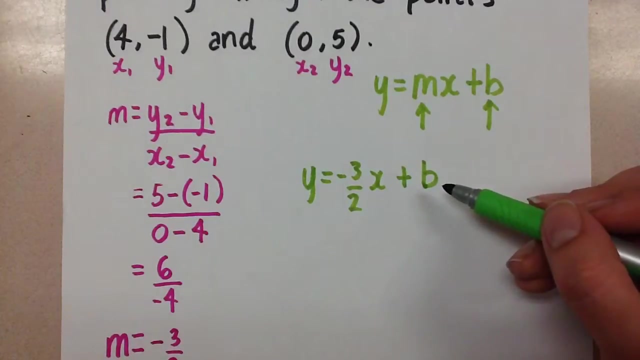 to finish the equation, Let's take this slope and plug it in to our equation. then y equals negative 3 over 2, x plus b. We need to find the b. That's what's missing for us now. We're going to use a point to do that. Either of the points will work if. 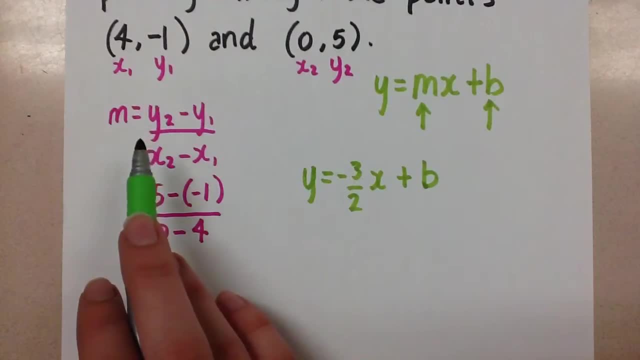 we do the calculations properly. It doesn't matter which point you choose. Both of these points are on the line, so they should give us the same y-intercept for that line. So when you choose a point, just make sure that you use the x and y values from the same point. 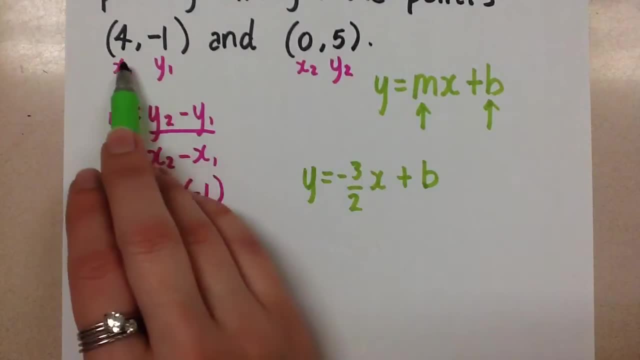 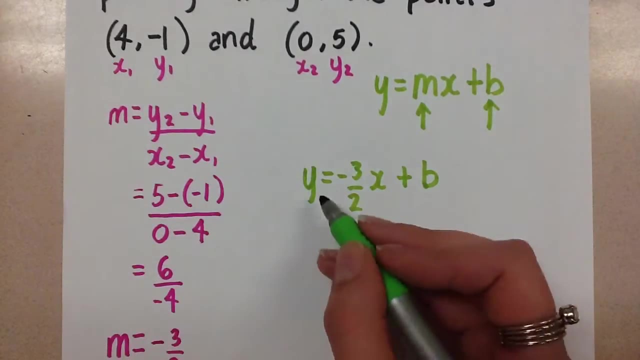 So if we choose this one, we'll use this x and this y, And if we choose this one, we'll use this x and this y. So we'll sub in the x and y values into the equation we're working with. So my y. 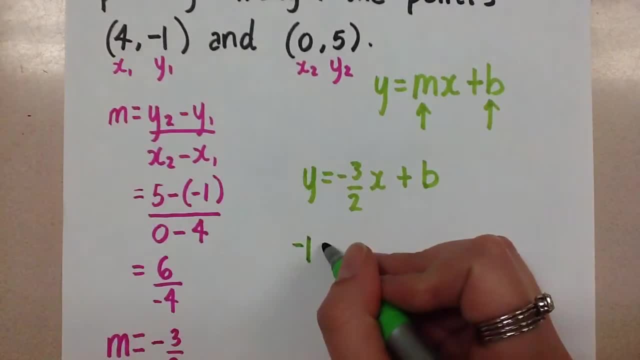 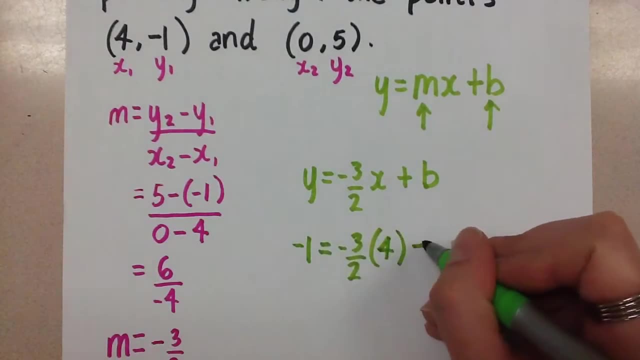 let's do this point is negative 1 and negative 3, over 2 times my x, which is 4, plus b. So here's our equation: The b is the unknown We want to solve for that b value. Let's multiply this. 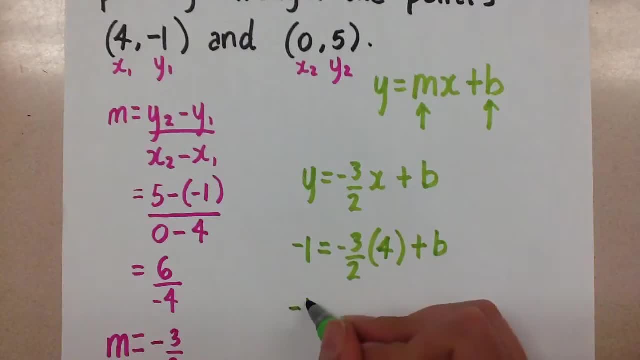 here. So we'll get negative 1 equals when you multiply negative 3 times 4 and then divide by 2, that gives us a nice whole number. That's negative 6 plus b, And now we want to move that negative 6. 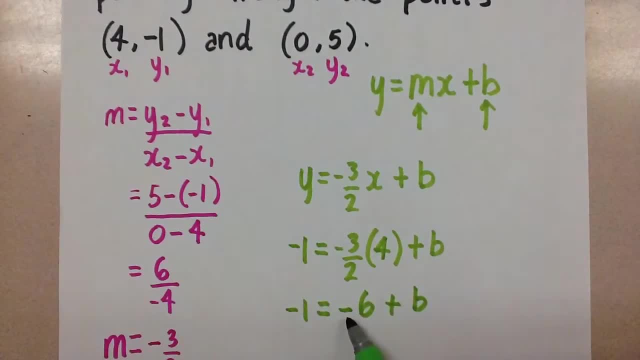 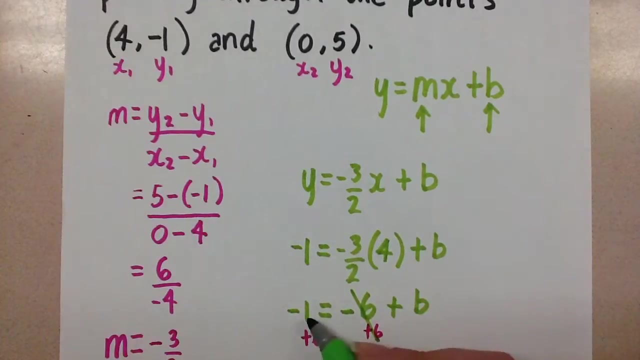 to the other side to get the b by itself. If it's minus 6 here we add 6 on both sides. That's the opposite, Opposite operation. So these cancel and we're left with: b equals negative, 1 plus 6 is positive.